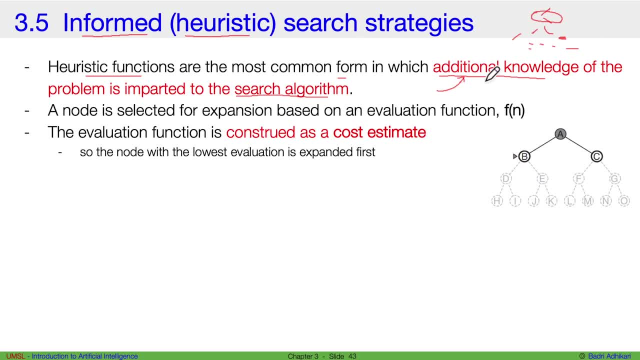 In case of informed search strategies, we want to inform the search algorithm to do lesser search so that the search can be faster and more effective, and we do this with the help of heuristic functions. Now, once again, all search algorithms, as I mentioned earlier, differ only in the way they select the next node for expansion. 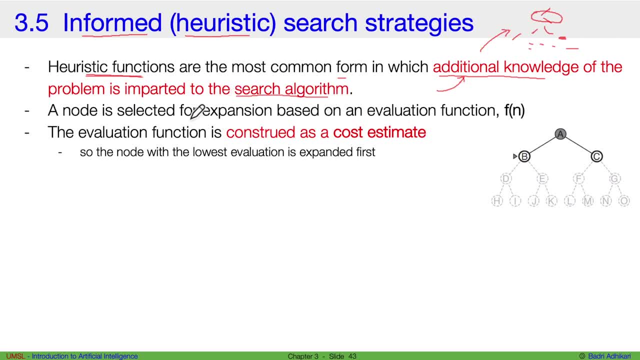 In case of informed search strategies, the node selected for expansion is based on evaluation function FN, And this evaluation function is construed as a cost estimate. So this gives you the estimate about the, or the idea of how far you are from the goal, And the node with the lowest evaluation is expanded first. 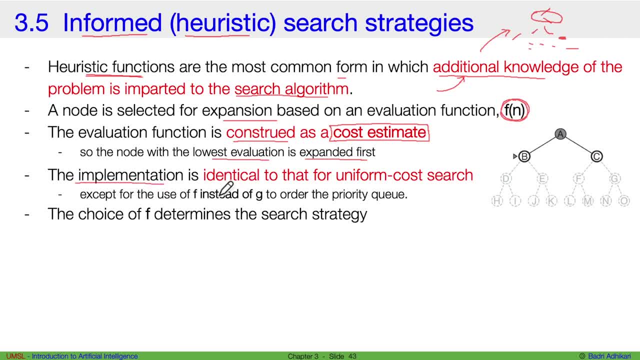 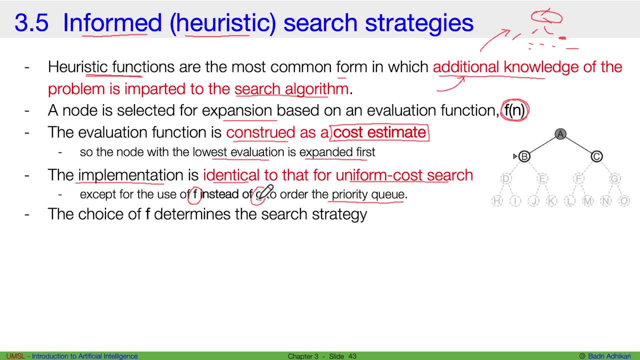 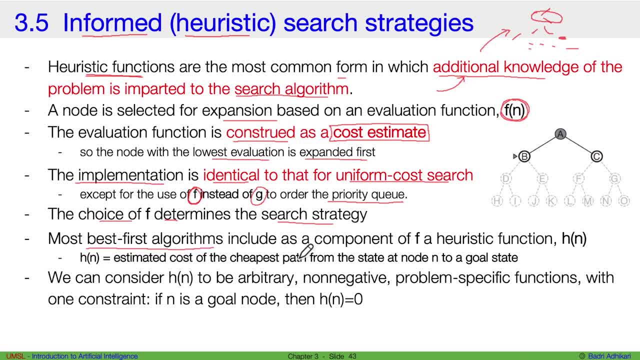 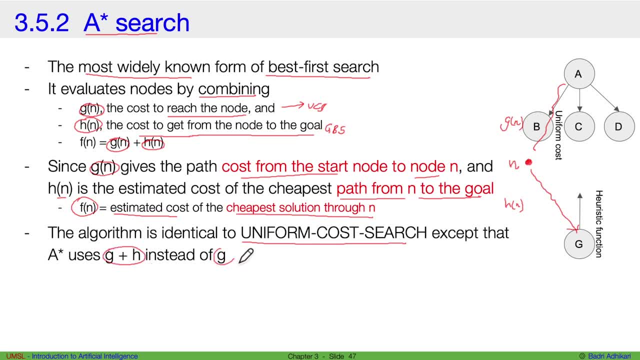 Now all the best forced search algorithms, which we will discuss one of them later, include, as a component of F, that is, this function, a heuristic function, this G plus H function, instead of just using G. Let us see how the A star search algorithm works. 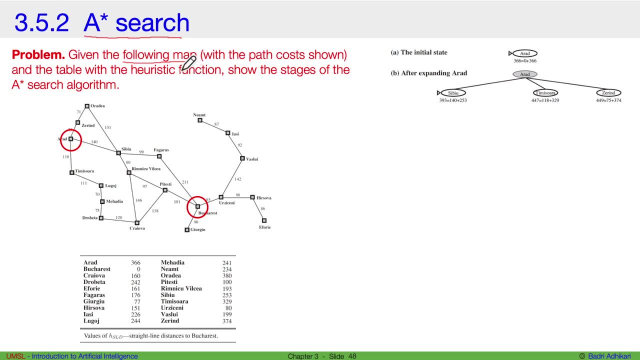 with an example Given the following map with the Romania problem with path cost shown in the map and a table given with the heuristic function. this is your HN table. we would like to see the stages of the A star search algorithm. 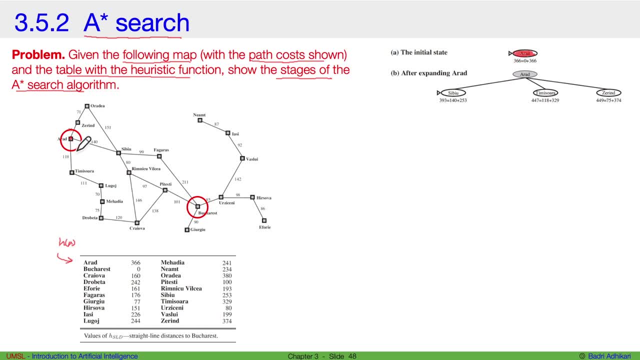 So we start with the city of Arad, our starting node, And the possible actions we can take are going to G, S and T, So we'll add these three cities into our priority queue: S, T and G. Now the values in the priority queue. 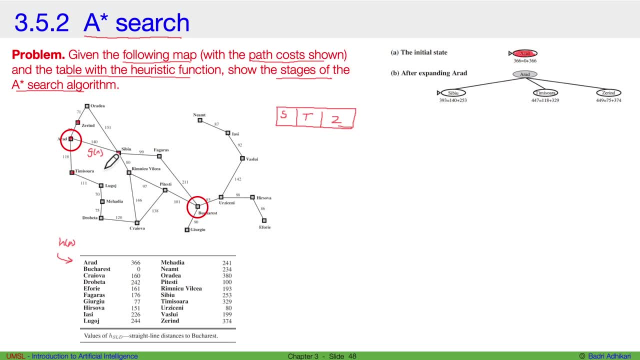 will depend on HN plus GN. So that means the priority for Timi Sota will be 118 plus HN of Timi Sota. So Timi Sota has a HN of 329.. 118 plus 329.. Similarly, the GN for Sibiu is 140.. 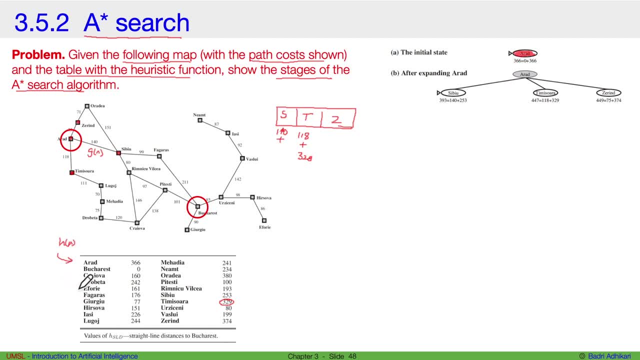 So the total priority or the total cost will be: HN for Sibiu is 253.. So it will be 140 plus 253.. Similarly, for Zerind, it will be 75 plus 374.. So this gives us these three possible nodes. 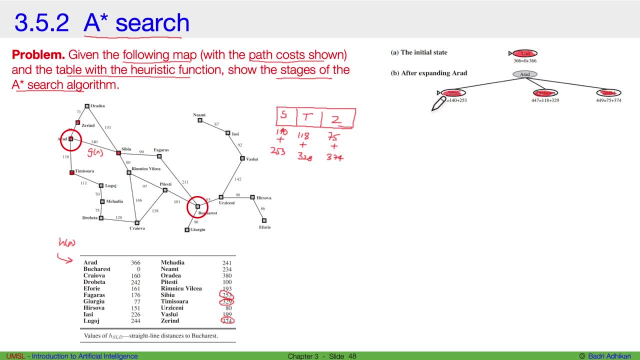 In the priority queue And out of these, since Sibiu has the minimum distance, minimum cost- 393- compared to two others, that is the next node that we will expand. So, after expanding Sibiu, the nodes that we have. 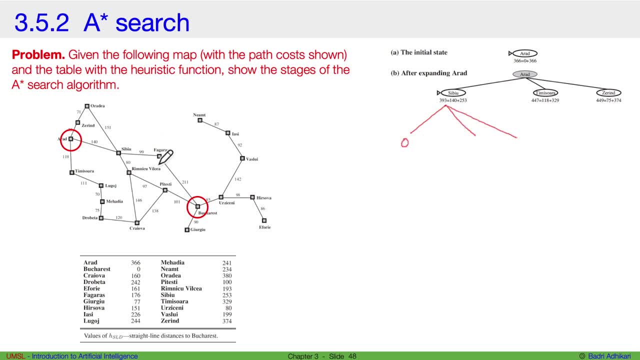 are the city of Oradea O another city, Faragas, and the city R. Now the costs associated with these cities are: the cost from Sibiu to Faragas is 140 plus 99,, 140 plus 99, plus the cost of going. 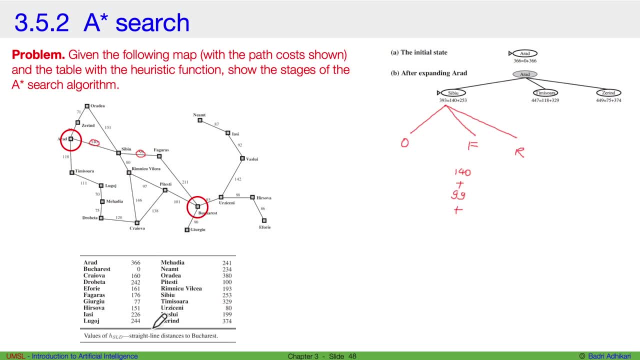 from Faragas to Bucharest. So Faragas to Bucharest is 176 plus 176.. Similarly, for Oradea, it will be 75 plus 71,, 75 plus 71, plus 380.. And for this city R, the cost will be 75 plus 71,, 75 plus 71,. 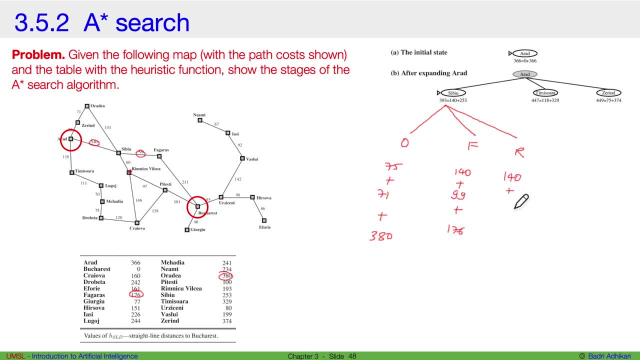 plus 380.. And for this city R the cost will be 75 plus 71,, 75 plus 71, plus 380.. And for this city R the cost will be 140 plus 180, sorry, only 80 plus 193.. 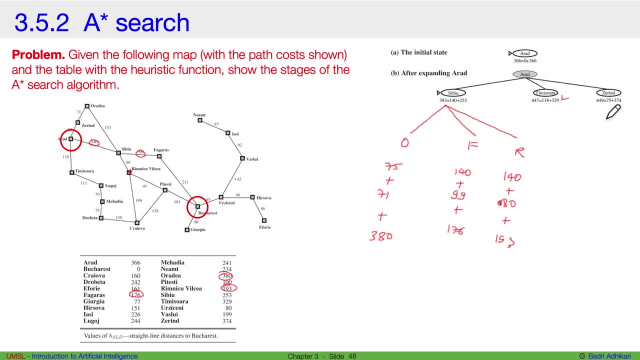 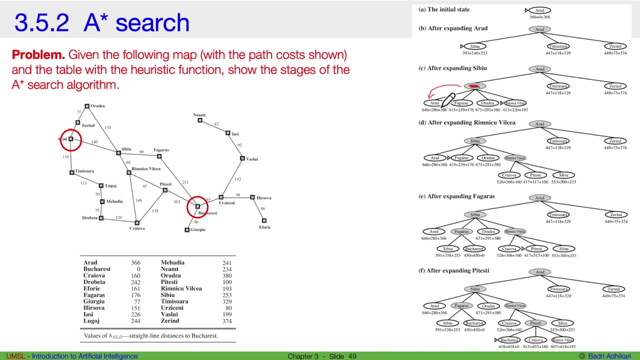 So now what we have in the priority queue is these two cities, along with these three cities, And whichever has the minimum cost out of all these cities is expanded. Here's a full solution that shows that from Sibiu, you can actually go back to Oradea as well. 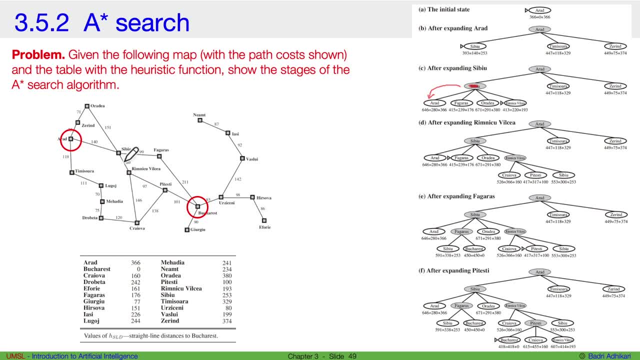 and then compute the paths. That is, after going to Sibiu you can go back to Areth with the cost of going here and then going back and then checking that. Usually that will not give you better solutions. So here's the cost of going to Faragas, Oradea and R. 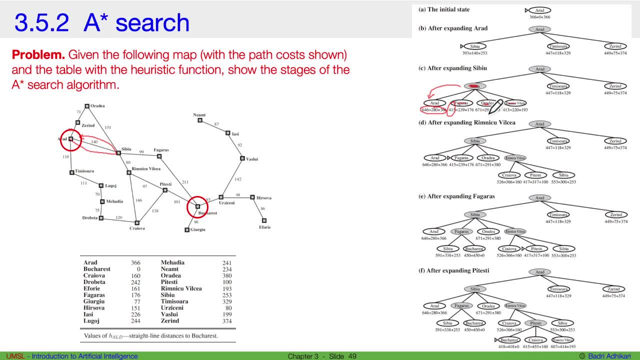 And we see that the priority queue now has 415F, 6710,, 413R and 447T and 449G. So out of these, since R has the minimum path cost, next we expand R. Now, then we have: 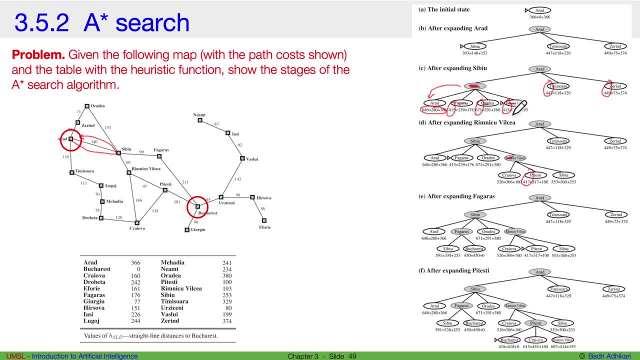 OK, Next subsequent nodes. So after expanding R, what we have is these additional nodes And we see that Faragas has the minimum total cost. So it will expand Faragas And we have Bucharest at a cost of 450.. It will next expand the next node, P, And then we 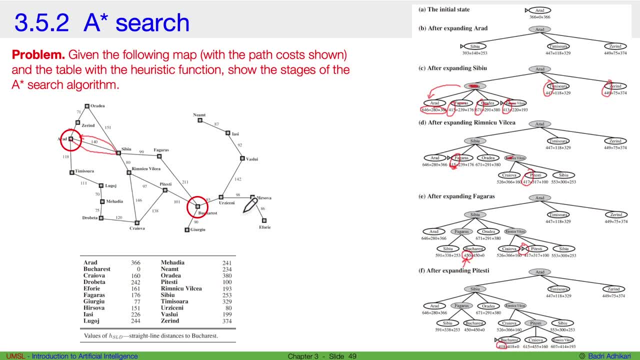 get to Bucharest again with even a lower path cost. that is, at first it goes through this path. The total cost is 450.. Then it tries the next path And that gives us 418.. So this is how the h-star algorithm works. 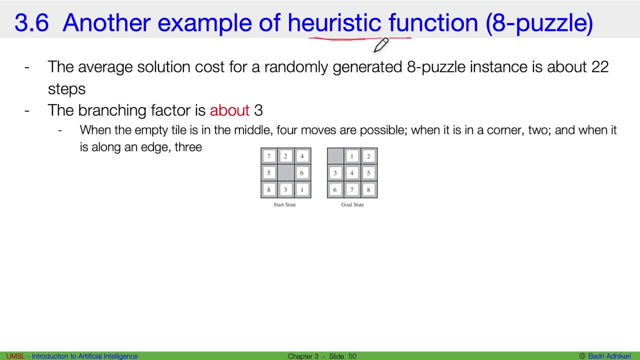 So heuristic functions are extremely powerful. Your immediate question may be for a given problem: how do I know what heuristic function to use? And the answer is: there is no formula. The only way to learn about heuristic functions is to look at examples. 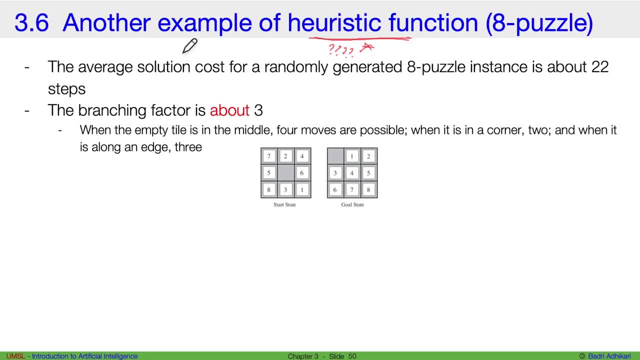 And use them as inductions to build your own heuristic functions. So let's look at another example of the heuristic function for the eight puzzle game. The average cost for a randomly generated eight puzzle instance is about 22 steps. In other words, you start from the first step. 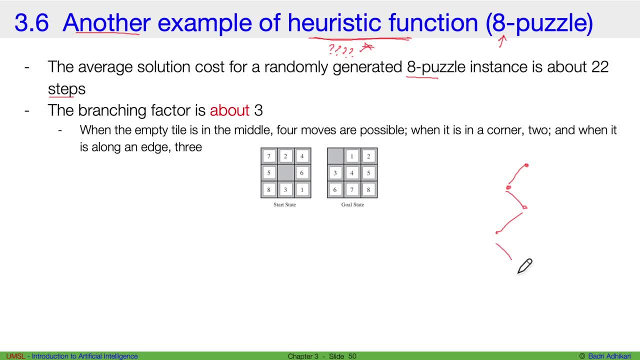 make random changes, make random changes again, make random changes again. So only after approximately around 22 steps will we find the actual solution, And the branching factor is about three. It's about three because, if you are here, you have four choices to make. 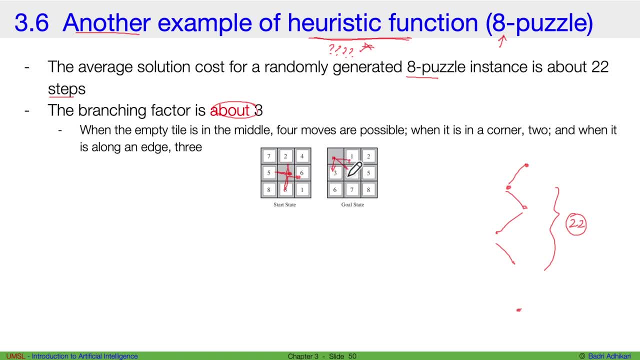 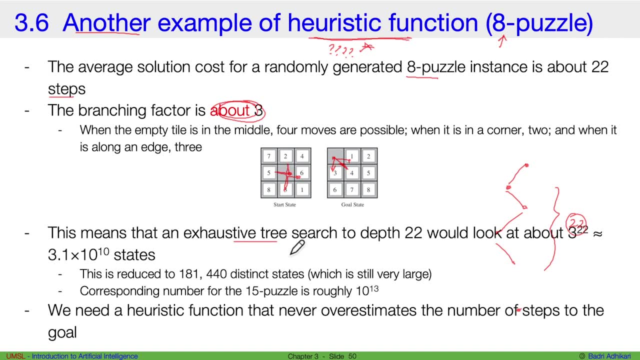 If you are here, you only have three choices to make, Only two choices to make. So on average, the branching factor is about three only. This means that an exhaustive tree search algorithm to depth 22 would look at about three to the power 22. 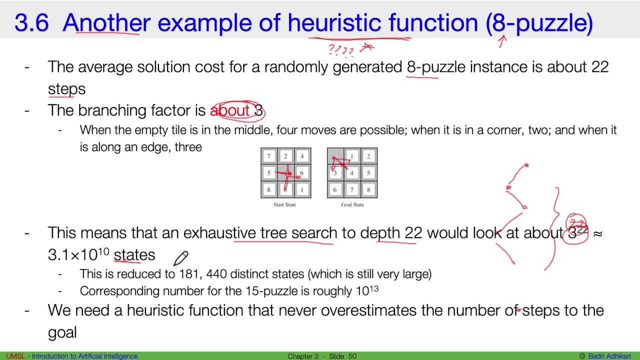 number of states, Given that there is only a few steps. that's the end of the question. fixed kinds of moves that we can do. this will reduce to around 181,000 distinct steps, which is still very large. Now, if we had the puzzle of a bigger size say, 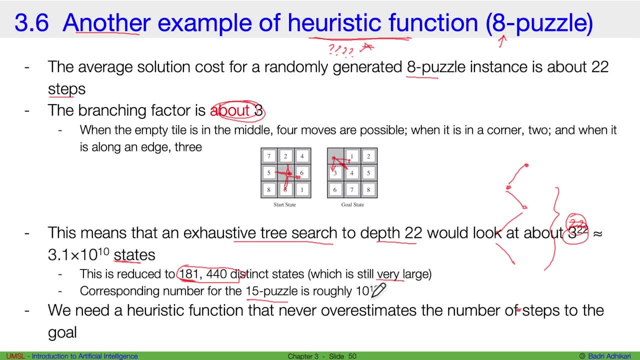 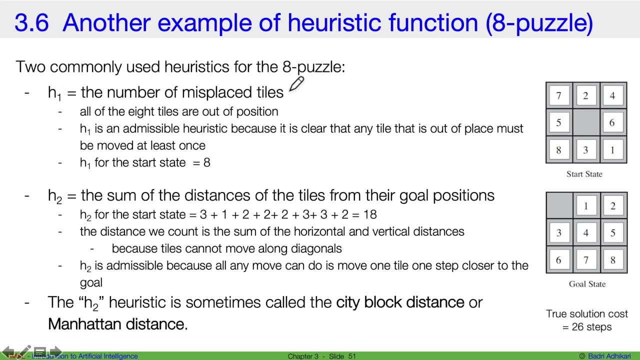 15 piece puzzle, then this number would roughly be a very, very large value. So we need a heuristic function that never overestimates the number of steps to the goal state For the eighth puzzle game. here are two commonly used heuristics: The: 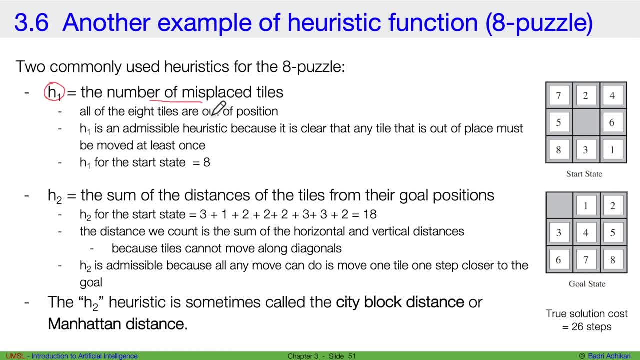 first one, known as H1, is the number of misplaced tiles. That is, what we look at is how many tiles are misplaced compared to the goal state. So here, if this is our starting state and if this is our goal state, the number of misplaced tiles. 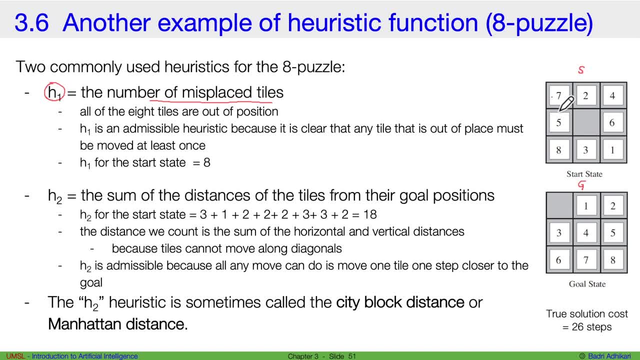 let's count them. So let's look at the first corner: 7.. Is 7 at the correct position? No, So one misplaced tile: Is 2 at the correct position? Another misplaced tile: Is 4 at the correct position? No, another misplaced tile: 5? No Blank, No 6? No 8? It's also not in the 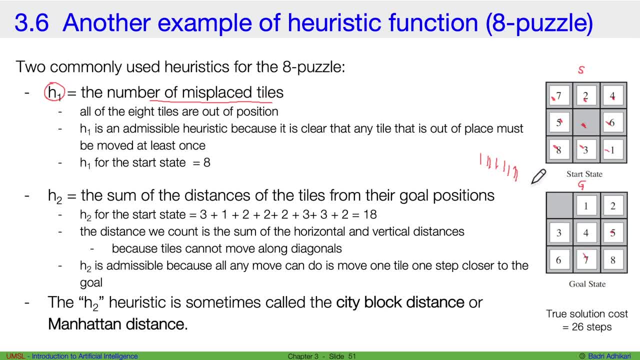 correct position? 3? Not 1? Not, So none of them are in the correct position. So the total cost is 1, 2, 3, 4, 5, 6, 1, 2, 3, 4, 5, 6, 7, 8, 9.. In other words, this node has this state. 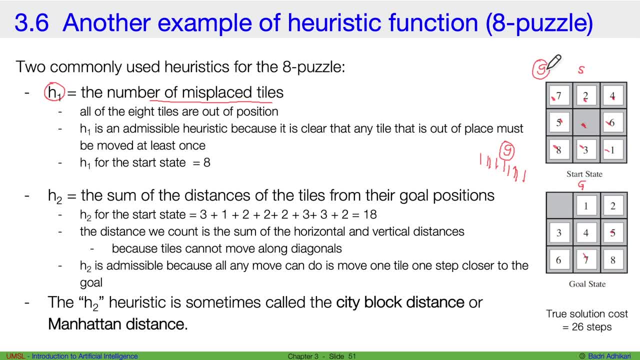 has a cost of 9,, which is the worst possible cost. Since all of the 8 tiles are out of position, we could say it's only 8 because we can ignore the blank, And H1 is admissible heuristic because it is clear that any tile out of place must be moved at least once. 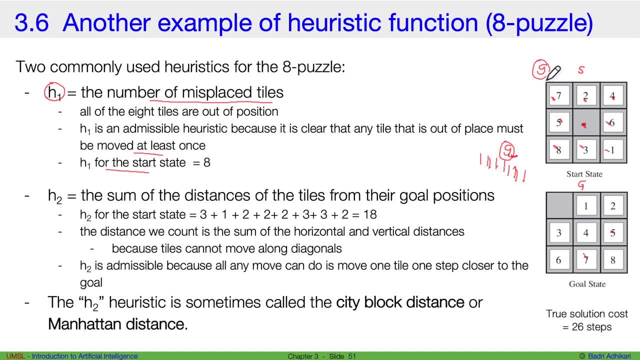 H1 for this state is not 9, but effectively 8, only ignoring the blank space. Next heuristic is H2.. This is the heuristic is also known as the city block distance or Manhattan distance. Here we look at the sum of the distances of the tiles from their goal. 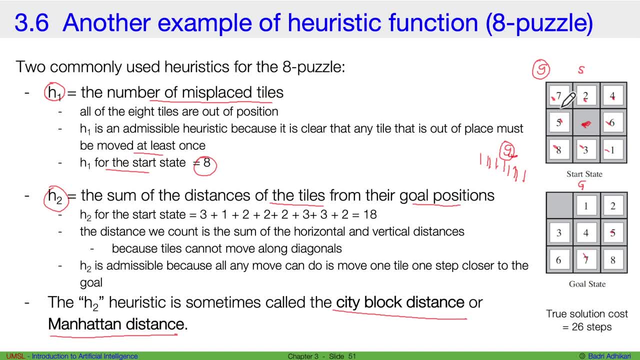 positions. What we look at is how far each tile is from where it should be. So if we look at this number 7, how far it is is it should be here, but it's there. So the distance is 1,, 2, and 3.. Distance is 3 for 7, plus. let's look at the second 2.. 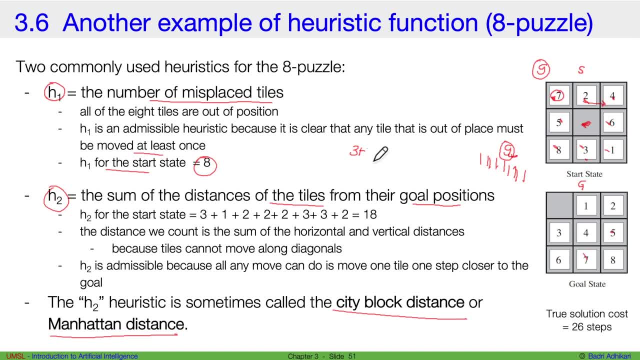 This block 2 should be over here, so it's one step far away. plus, this block 4 should be 1, 2 blocks away, 2.. This is what you see here. So in this way, if you sum up the distances, 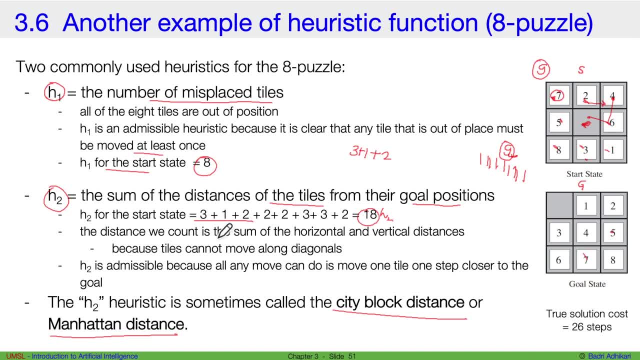 from each node. what you get is your H2 heuristic. So obviously, higher the distance, the worse your state is. The lower the distance, the better your state is. The distance we count is the sum of the horizontal and vertical distances, because we cannot move along the